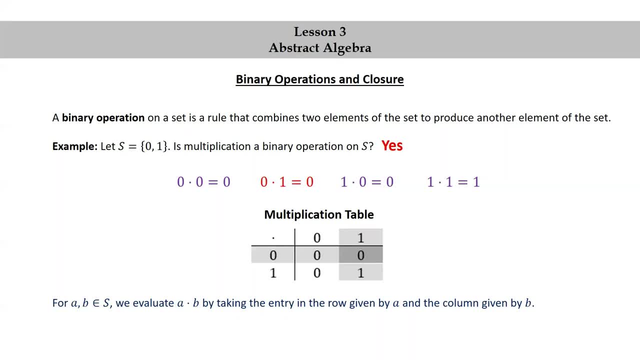 This shows us that 0 times 1 is equal to 0. I would recommend pausing the video for a moment at this point and making sure you understand how the other three computations work using this multiplication table. 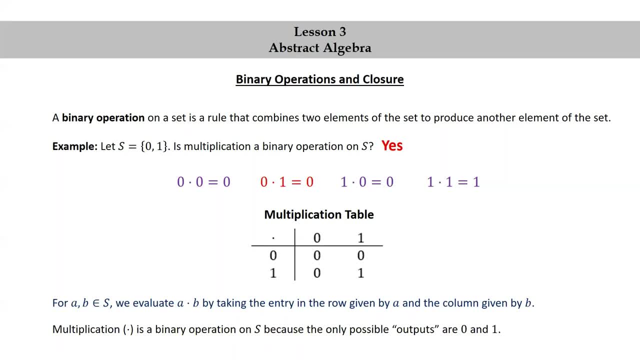 Multiplication is a binary operation on the set S because the only possible outputs are 0 and 1. for mostillah We see here that there are two inputs 0 and 1, and there are four outputs, but all four of those outputs are 0's and 1s. 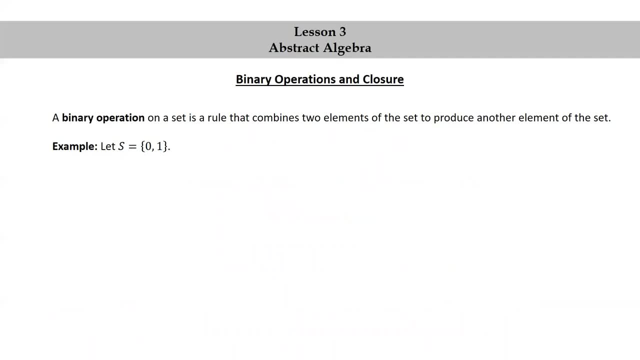 while it clearly explains the case when functions and all boundary inputs north, south and south occur together. Let's look at another example. We'll use the same set. S is equal to the set consisting of 0 and 1. b is equal to the set consisting of 0 and 1. Let's very clearly explain the processing technique that satellites and other Mes结 뭐가+. together. This time, we assist the group to now go to airplane下面 to execute a yourselves passes~! An example bring up four inputs in the model into the array here. performance classes and süma tree of summer days come to the assignment setting that is feelings to things such as use ark parfait cell 알�ler and Warrior arranging generals fillages are Trad surgery skills to other friends. After All, we review what a particular component is about high university 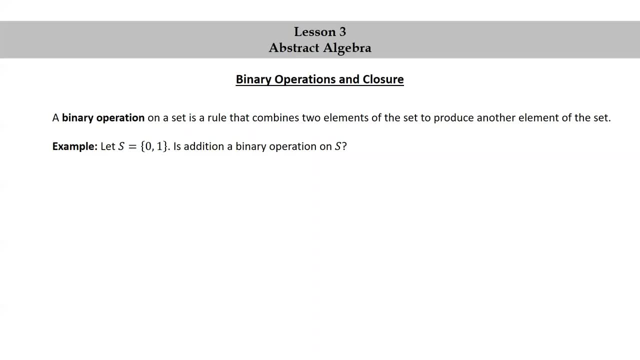 question is addition a binary operation on the set S? Well let's do the four computations. 0 plus 0 is equal to 0, that one's okay. 0 plus 1 is 1, that's okay. 1 plus 0 is equal to 1, also okay. 1 plus 1 equals 2, that's not okay because 2 is not in the original set S, so the answer is no. Once again the problem is that 1 plus 1 is equal to 2, and 2 is not an element of the set S. Let's look at the multiplication table for this example. We see here the problem is that the inputs are 0 and 1 but there's an output of 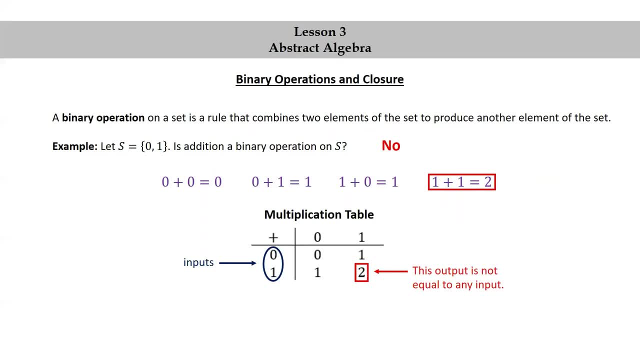 2 or 1. That's not true in the Set S syntax. It's totally okay, but we'll talk an which is not equal to either of those inputs. 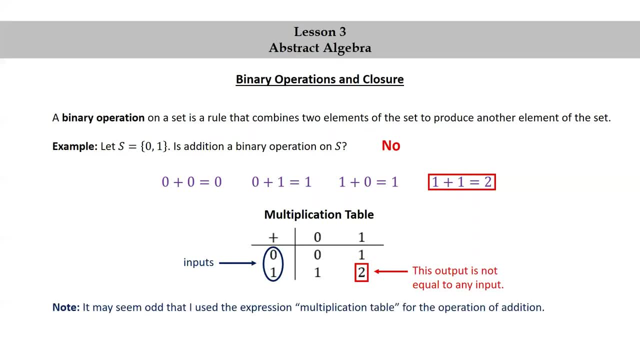 Note, it may seem odd that I use the expression multiplication table for the operation of addition. Nonetheless, multiplication table is a general expression that can be used for the table describing any binary operation, or any operation at all. 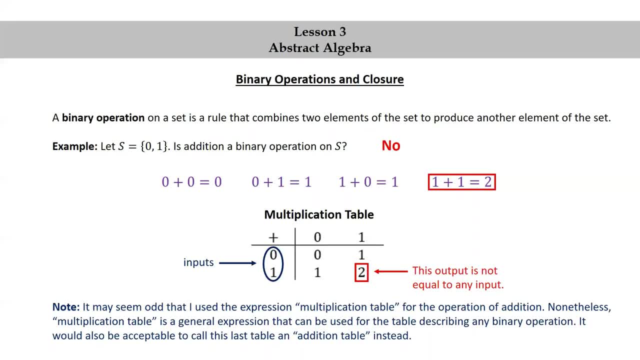 It would also be acceptable to call this last table an addition table instead. 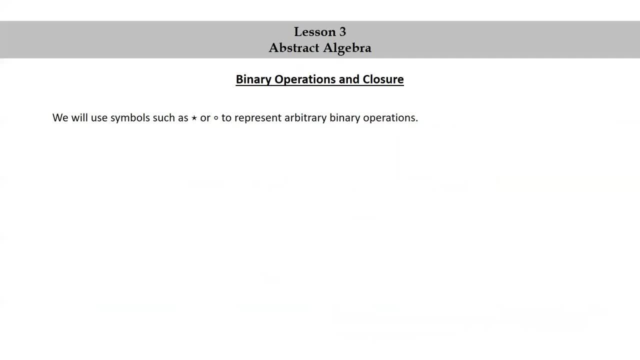 We will use symbols such as star or dot to represent arbitrary binary operations. If the binary operation is one that we are familiar with, then we will use the appropriate symbol. For example, we will use the symbol plus when the binary operation is addition. 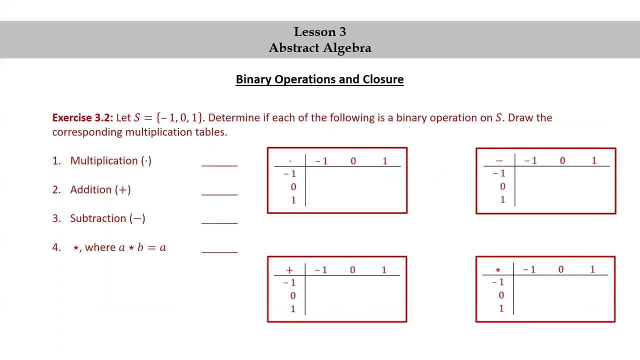 Let's try an exercise. Let S be the set consisting of negative 1, 0, and 1. Determine if each of the following is a binary operation on S, and draw the corresponding multiplication tables. 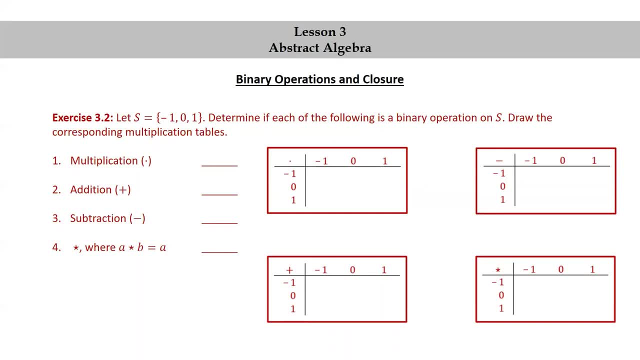 Now is a good time to pause this video, try this problem yourself, and then resume the video to check your answers against mine. 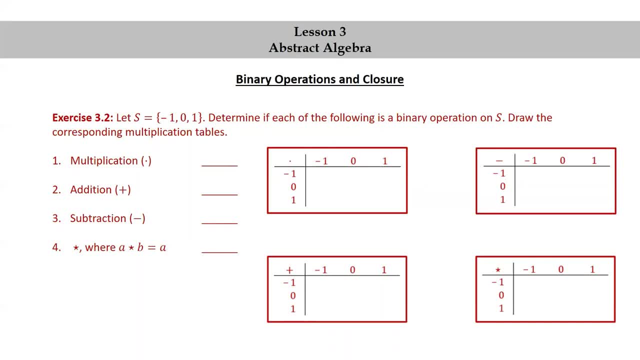 Okay, the first one is multiplication. Let's look at the table for multiplication. And we see that all the outputs are 0s, 1s, and negative 1s. 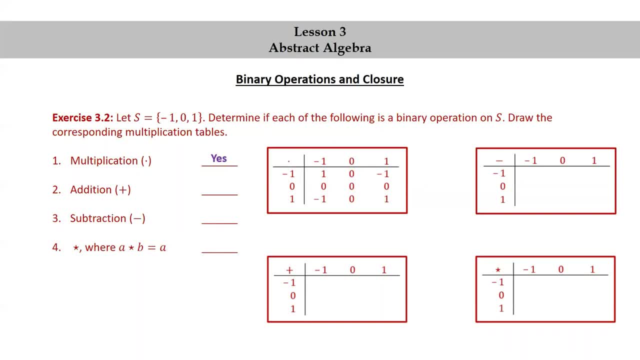 So yes, multiplication is a binary operation on this set S consisting of negative 1, 0, and 1. 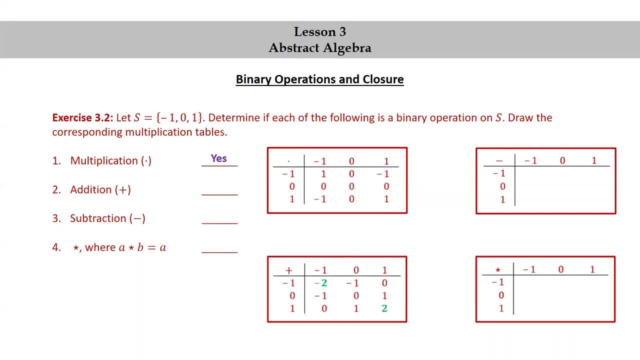 Next we have addition. If we look at the set S, we will see that S is a binary operation. If we look at the multiplication table for addition, or equivalently the addition table, 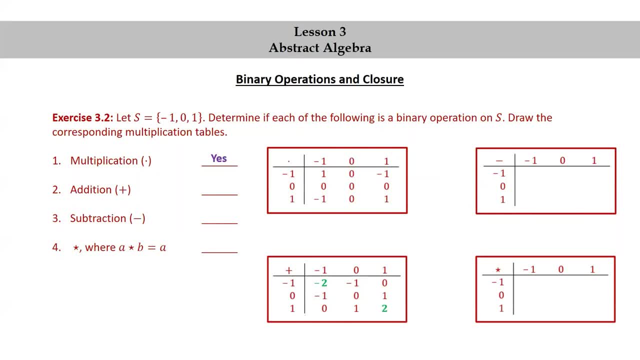 then we see that there's a 2 and a negative 2 in there. Both of those cause a problem, which means that the answer is no. 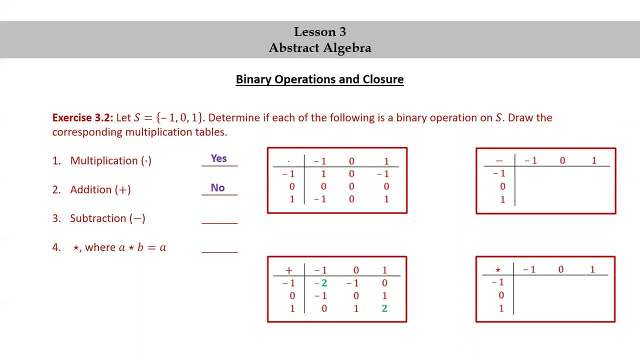 Addition is not a binary operation on this set S consisting of negative 1, 0, and 1. 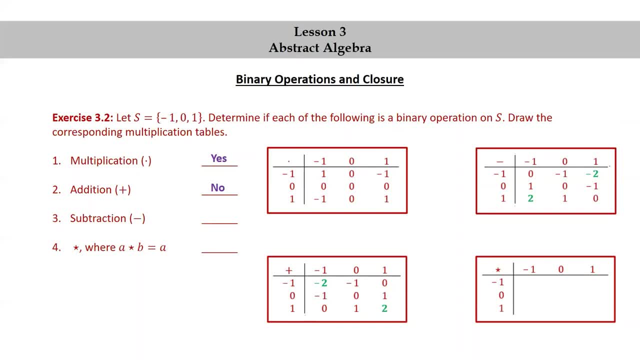 The next one is subtraction. The multiplication table for subtraction, or equivalently the subtraction table, also has some problems. 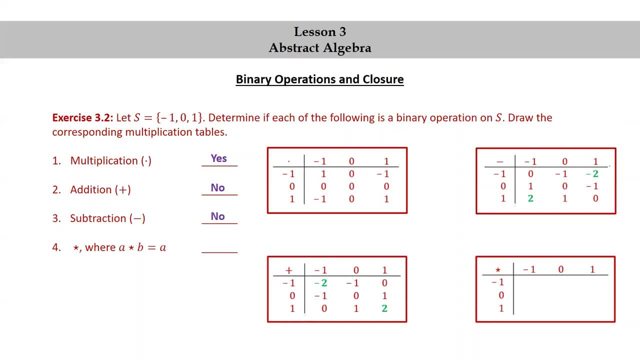 There's a 2 and a negative 2 in there as well, so the answer is also no. 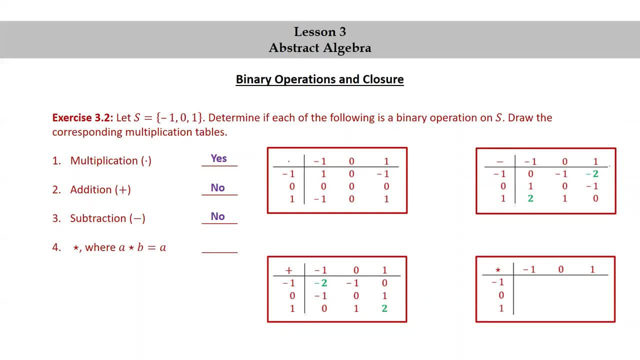 Subtraction is not a binary operation on the set S consisting of negative 1, 0, and 1. 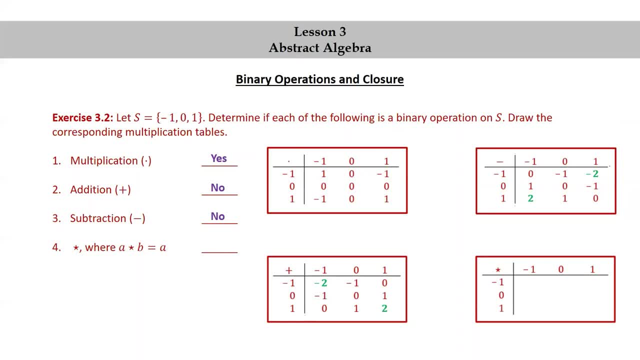 For the last one, we have star, where a star b is equal to a. In this case, the output a is equal to one of the given inputs. So the answer is yes. 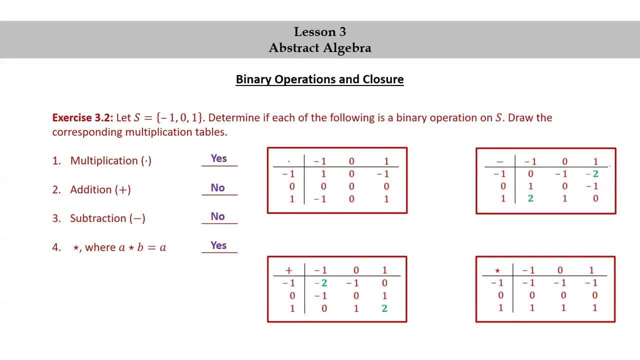 This operation star is a binary operation on the set S. 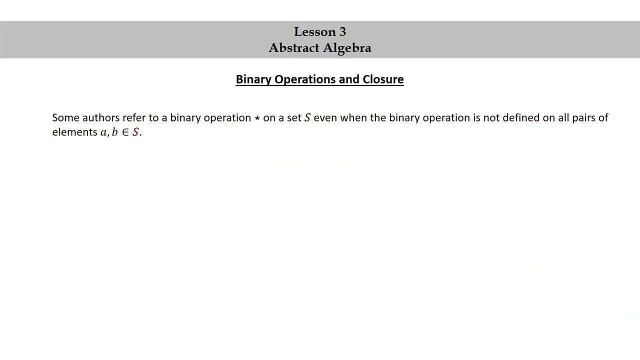 Some authors refer to a binary operation star on a set S even when the binary operation is not defined on all pairs of elements a, b, and s. We will always refer to these false operations as partial binary operations. 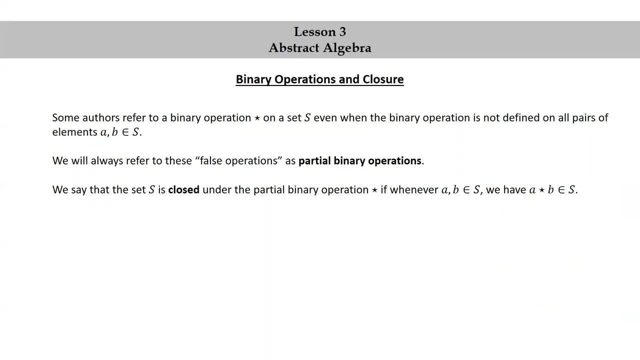 We say that the set S is closed under the partial binary operation star if whenever a and b are in S, we have a star b in S. 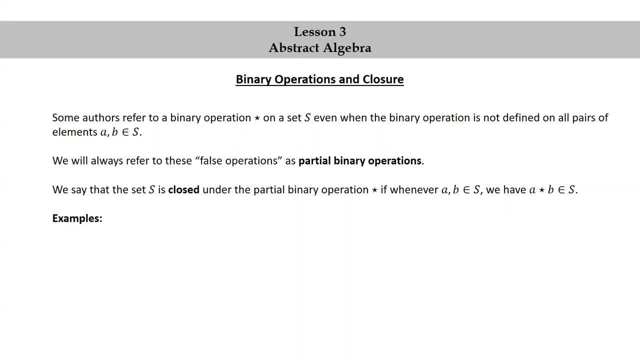 Let's look at some examples. The set consisting of 0, 1 is closed under multiplication. This is just another way of saying that multiplication is a binary operation on the set consisting of 0 and 1. 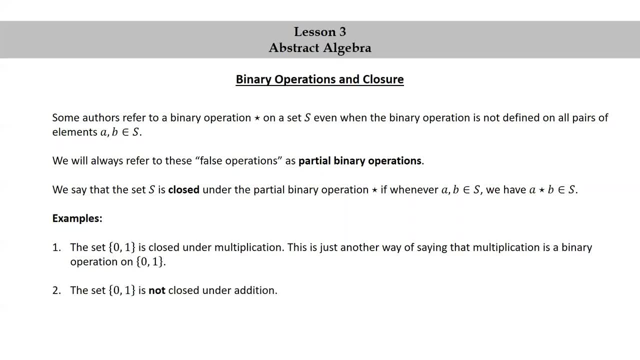 The set 0, 1 is not closed under addition. In other words, addition is a partial binary operation on set 0, 1 that is not a binary operation on set 0, 1. Let's try another exercise. 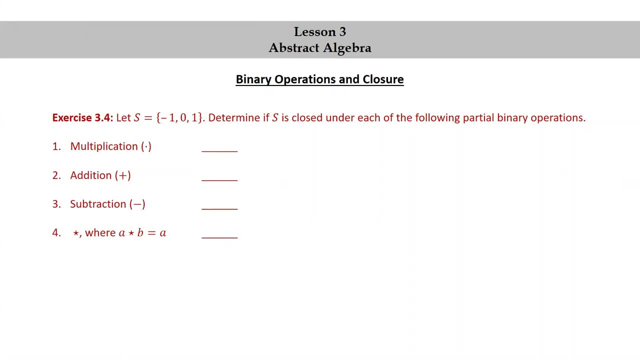 Let S equal the set consisting of negative 1, 0, and 1. 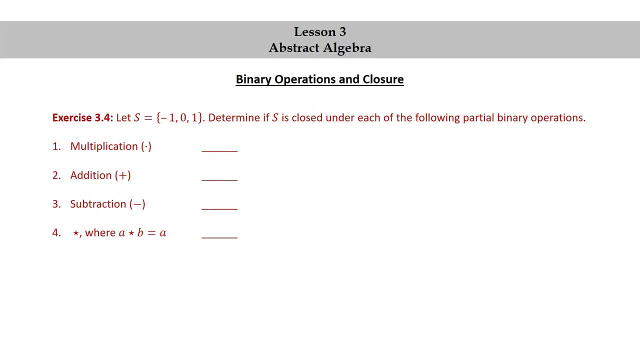 Determine if S is closed under each of the following partial binary operations. Now is a good time to once again pause the video, try this exercise yourself, and then resume the video to check your answers against mine. 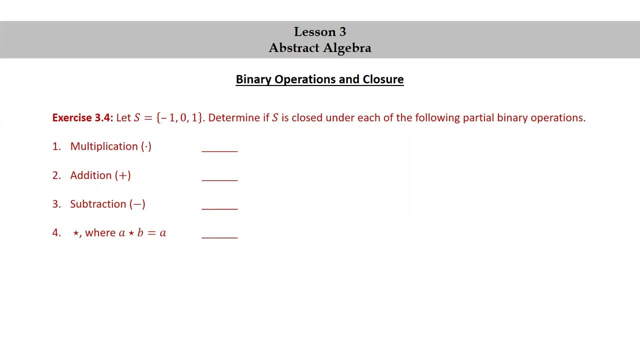 This question is actually asking the same thing as we have asked in the previous exercise. First, let me put down all of the multiplication tables that we already drew. For number one, multiplication. Is the set S closed under multiplication? Yes. 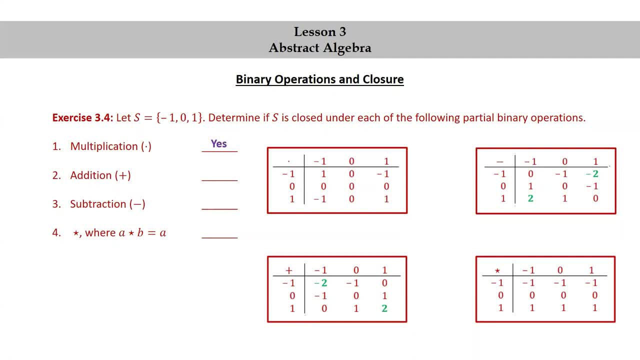 That's the same thing as asking if multiplication is a binary operation on S, and we already answered that. The same goes for the rest of them. 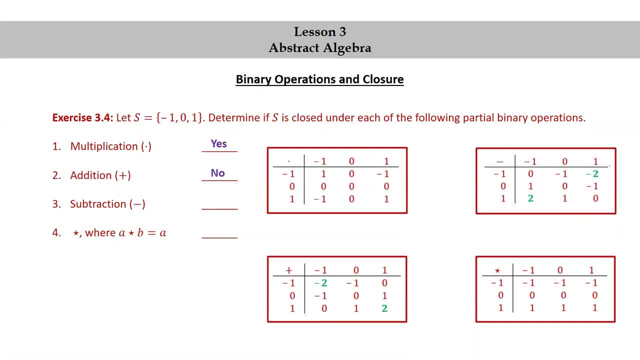 S is not closed under addition. It's not closed under subtraction. 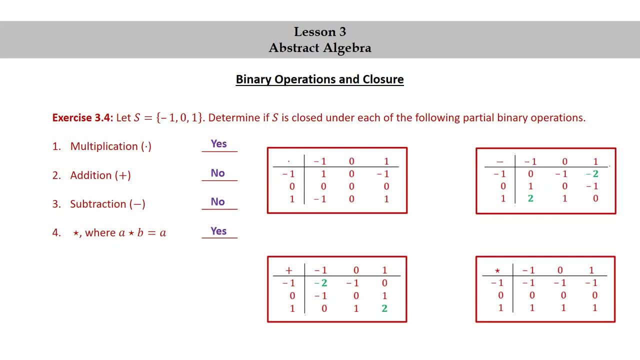 And S is closed under the operation star, where a star b is equal to a. 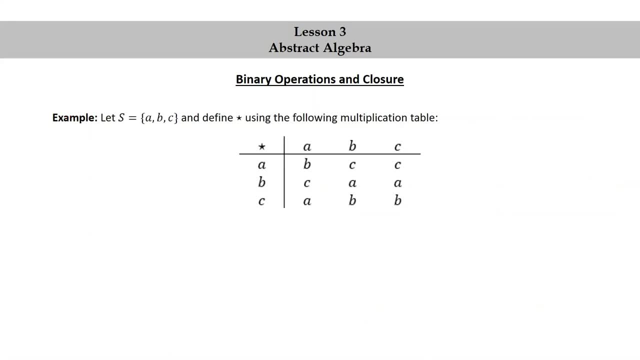 Let's look at another example. Let S be the set consisting of a, b, and c, and define star using the following multiplication table. 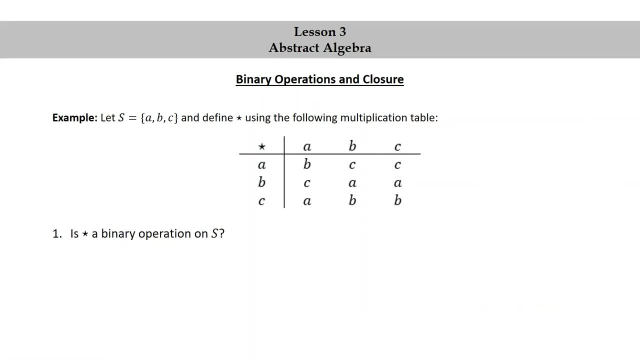 Is star a binary operation on S? Well, notice that all of the outputs are either a's, b's, or c's. So the answer is yes. 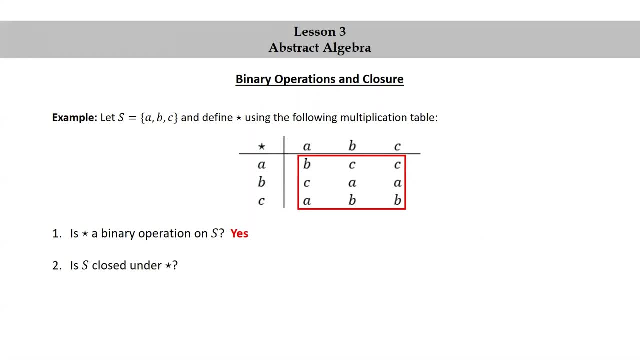 Is S closed under star? That's just another way of asking the same question. So the answer is yes. 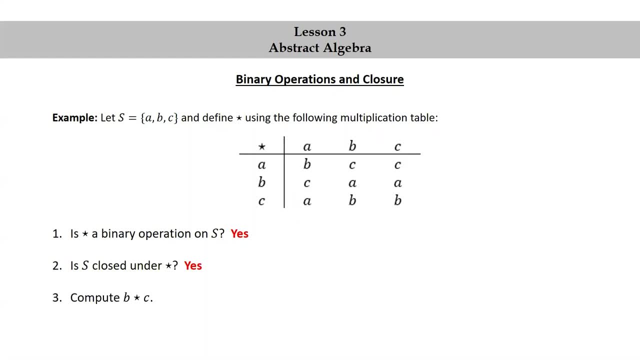 Compute b star c. Okay, so for this, we look at the entry in the row given by b and the column given by c. 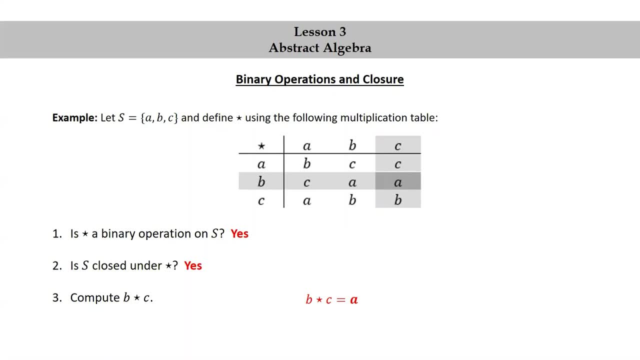 So we see that b star c is equal to a. 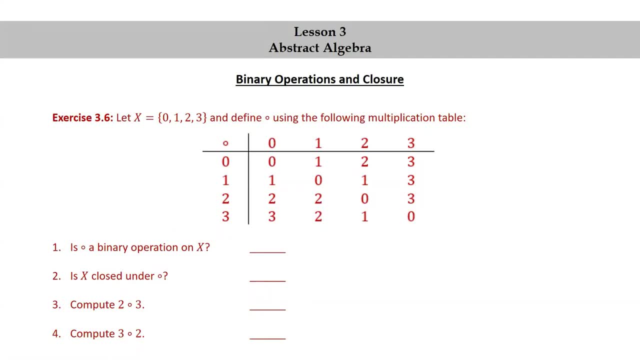 Let's try another exercise. Let X equal the set consisting of 0, 1, 2, and 3, and define dot using the following multiplication table. 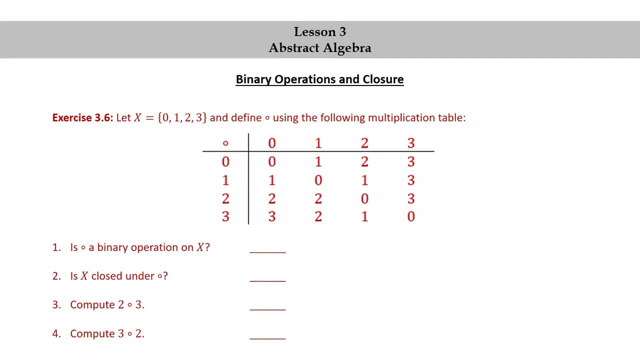 Is dot a binary operation on X? Is X closed under dot? Compute 2.3, and compute 3.2. 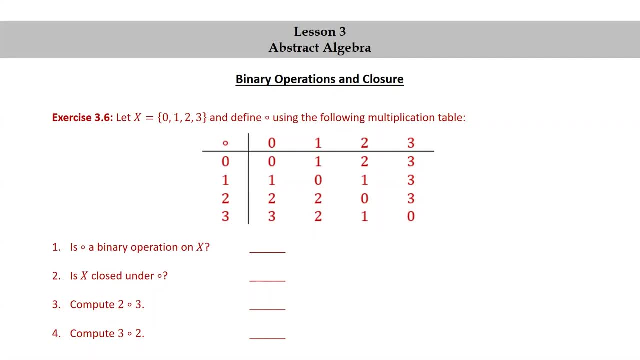 Okay, now's a good time to pause the video, try this exercise yourself, and then resume the video and check your answers against mine. Okay, so is dot a binary operation on X? Well, if we look at all the possible outputs, they're all 0s, 1s, 2s, and 3s. So, yes. Is X closed under dot? Again, yes. 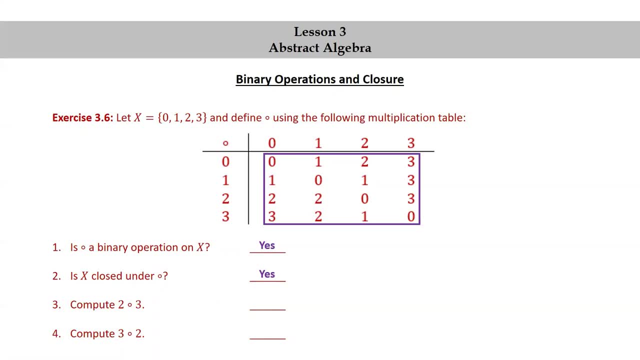 That's just another way of asking the same question as in number one. 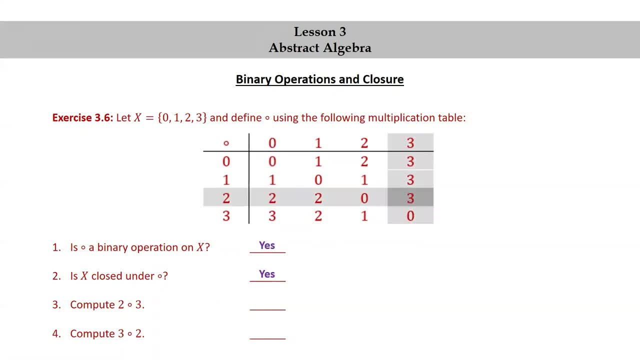 Compute 2.3. Okay, we look at the entry in the row corresponding to 2 and the column corresponding to 3. And we see that the answer is 3. 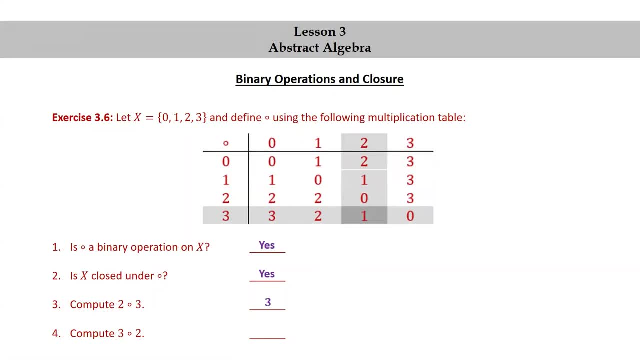 Compute 3.2. This time we look at the entry in the row corresponding to 3 and the column corresponding to 2. 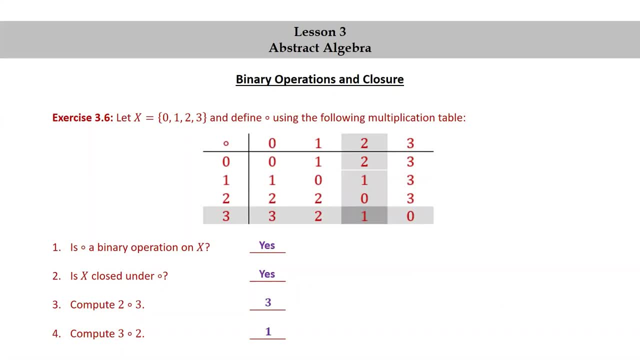 And we see that the answer is 1. 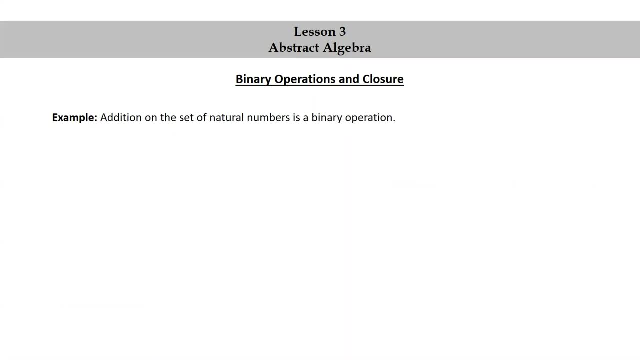 Let's look at another example. Addition on the set of natural numbers is a binary operation. 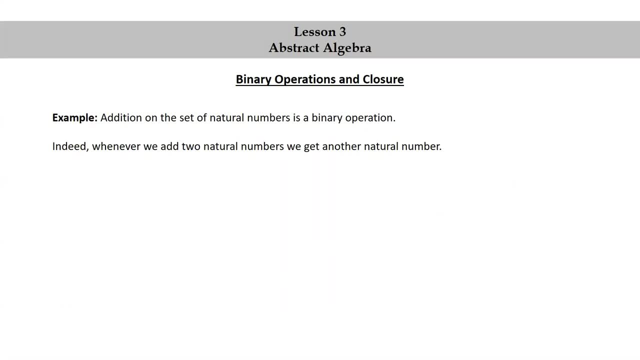 Indeed, whenever we add two natural numbers, we get another natural number. If a is a natural number and b is a natural number, then a plus b is a natural number. Equivalently, the set of natural numbers is closed under addition. Here is what the multiplication table or addition table looks like for addition on the set of natural numbers. The ellipses in the table indicate that we continue to increase each entry by one as we move to the right and as we move down from one entry to the next. As an example, to compute 1 plus 2, we look at the entry in the row corresponding to 1 and the column corresponding to 2. 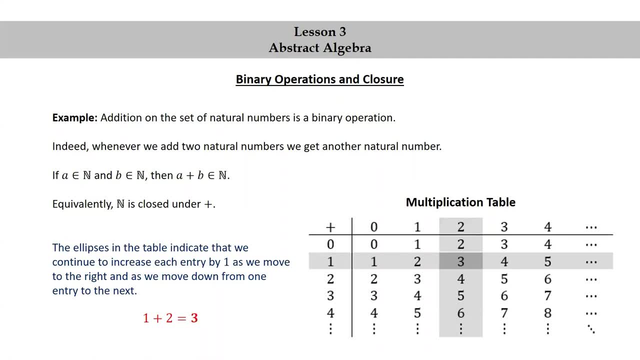 And we see that we get the number 3, which is what we would hope for. Another example. 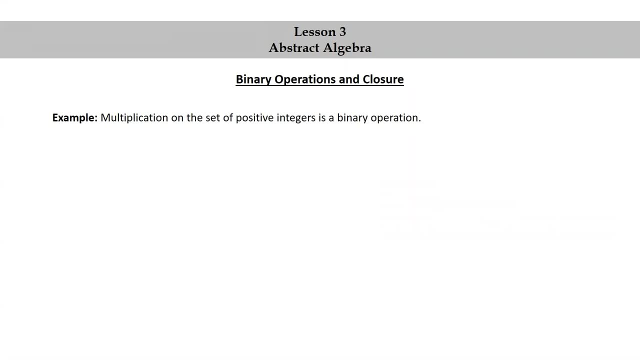 Multiplication on the set of positive integers is a binary operation. 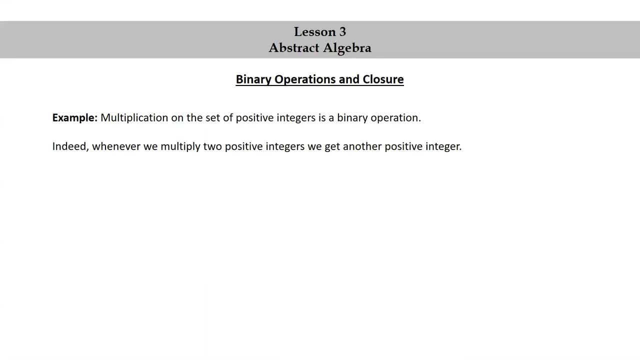 Indeed, whenever we multiply two positive integers, we get another positive integer. If a is a positive integer and b is a positive integer, then a times b is a positive integer. Equivalently, the set of positive integers is closed under multiplication. 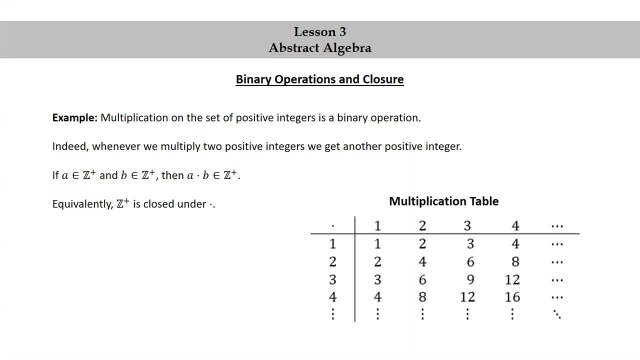 Here is the multiplication table. Equivalently, the set of positive integers is closed under multiplication. As an example, to compute 3 times 4, we look at the entry in the row corresponding to 3 and the column corresponding to 4. And we see that we get 12, which again is what we would hope for. Another example. Let s be the set of integers. 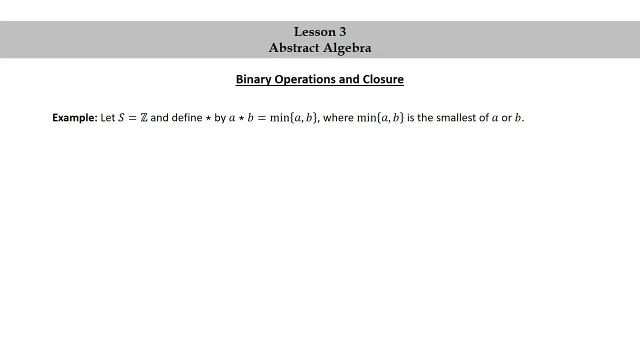 We find star by a star b equals min ab, where min ab is the smallest of a or b. Then star is a binary operation on the set of integers. Equivalently, the set of integers is closed under star. As an example, negative 5 star 3 is negative 5, because negative 5 is the smaller of the two numbers negative 5 and 3. Here is what the multiplication table looks like for this operation. Notice we have lots of ellipses here, because the set z goes infinitely from left to right. And if we write z going downwards, then it goes infinitely up and down. Another example. 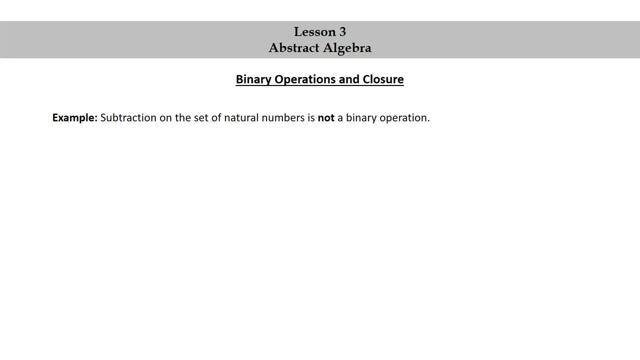 Subtraction on the set of natural numbers is not a binary operation. 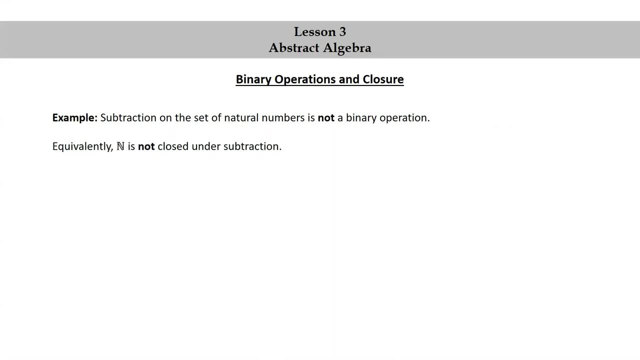 Equivalently, the set of natural numbers is not closed under subtraction. To see this, we just need to provide a single counterexample. A counterexample is an example that is used to show that a statement is false. For our counterexample, we could use 1 minus 2. 1 minus 2 is not an element of the set of natural numbers. Another exercise. 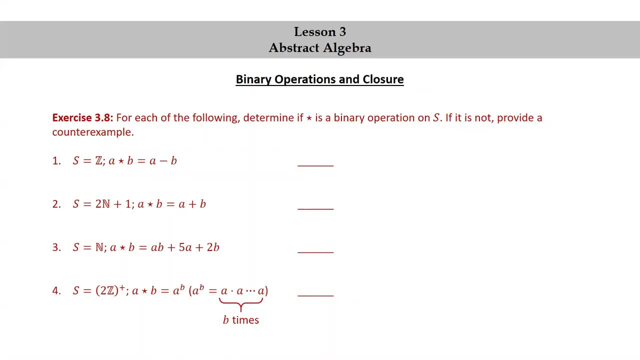 For each of the following, determine if star is a binary operation on s. If it is not, provide a counterexample. 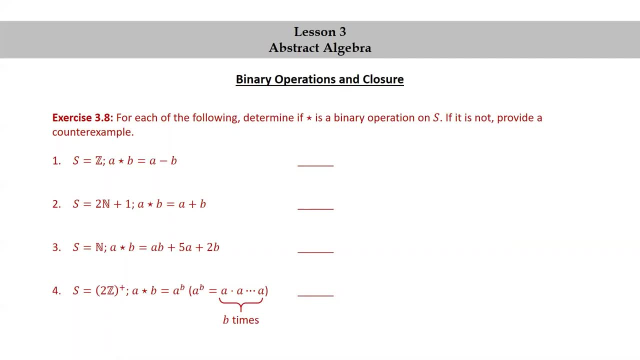 Once again, you should now pause the video, try this exercise yourself, and then resume the video to check your answers against mine. 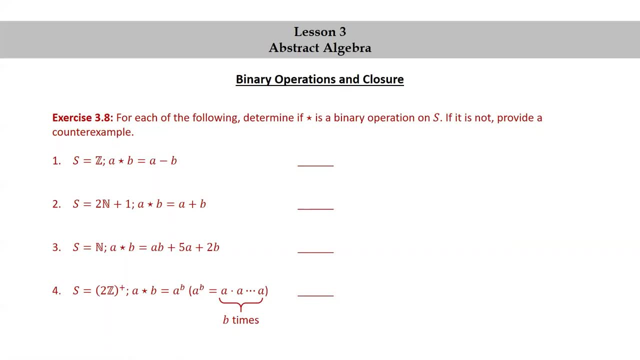 The first one. The set s is equal to z, the set of integers. 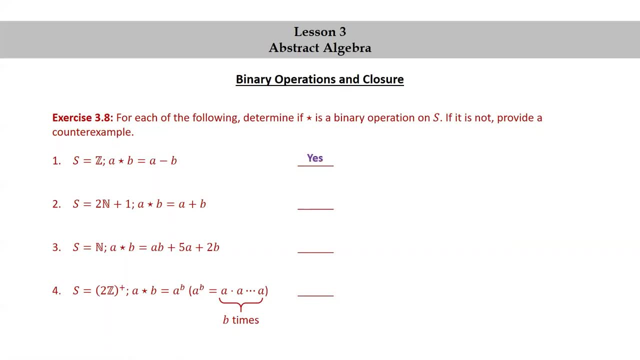 And a star b is a minus b. The answer to this is yes. Subtraction is a binary operation on the set of integers. Whenever you subtract two integers, you do get an integer. s equals 2m plus 1. That's the set of odd natural numbers. And a star b is equal to a plus b.